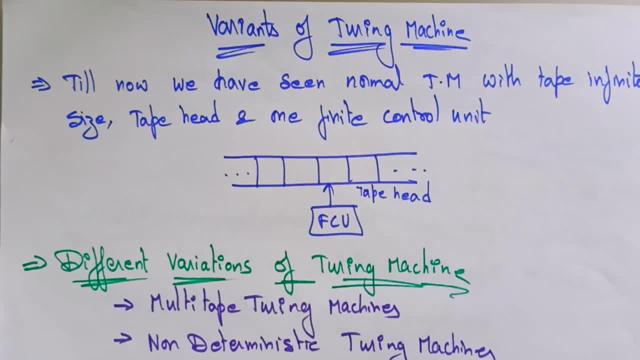 Hi students. coming to the next topic in the subject, theory of computations, is the variance of Turing machine. So far we have discussed about the Turing machine. Now let's see what are the different variables in the Turing machine. The variance or variations, whatever it may be. the same concept is the same, You can call. 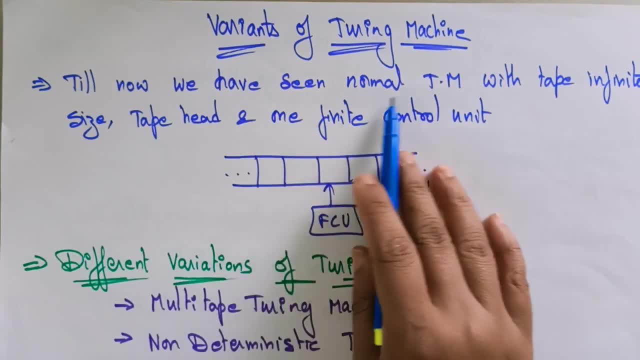 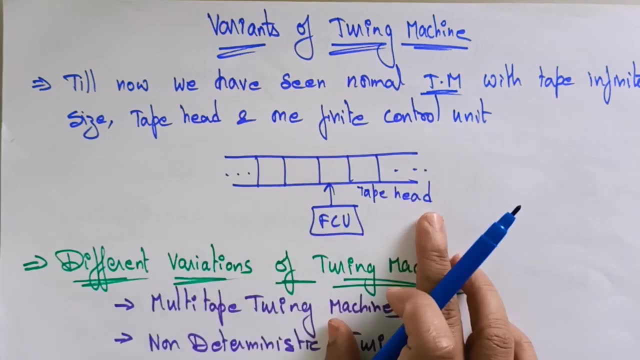 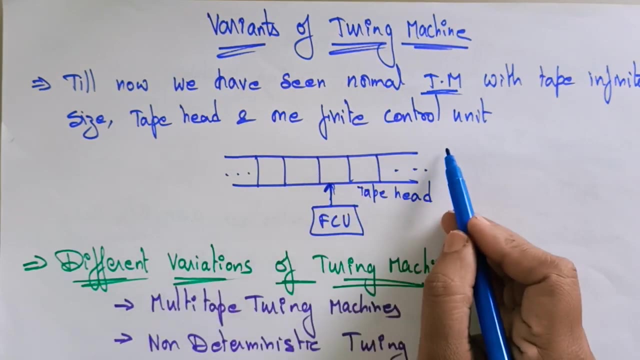 variations or variants. So till now we have seen normal Turing machine, Okay, the normal Turing machine with a tape of infinite size. So this is a tape with an infinite size which has the tape head, So this is a head that moves to the left or to the right, and one finite control unit. 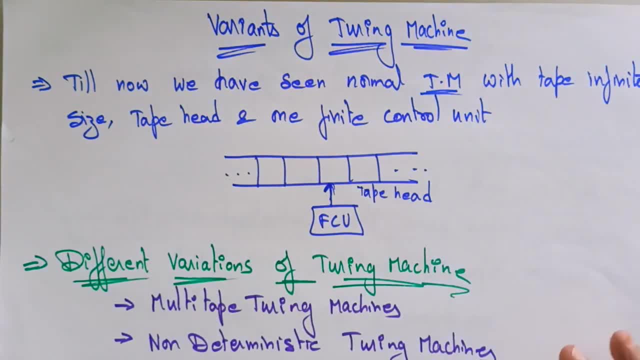 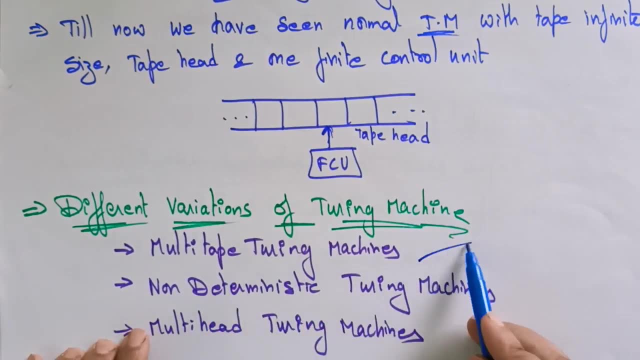 So far we learned about this Turing machine. Now let's see what are the different variations of the Turing machine. The different variations of Turing machines are: multi-tape Turing machine means there is a chance you can add the multiple tape. Here we have taken only one tape. 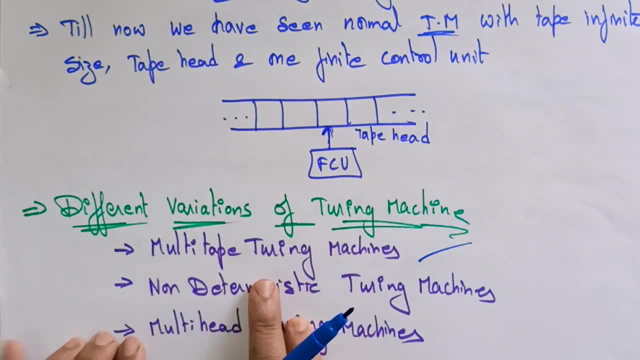 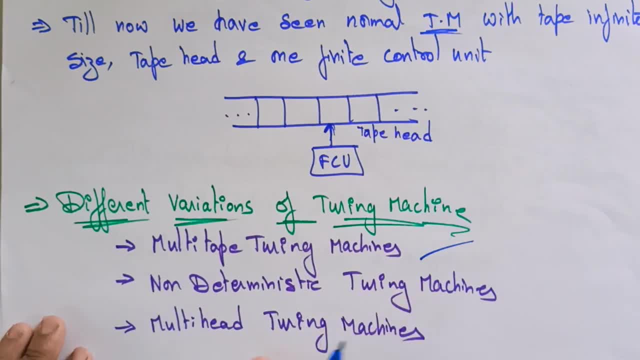 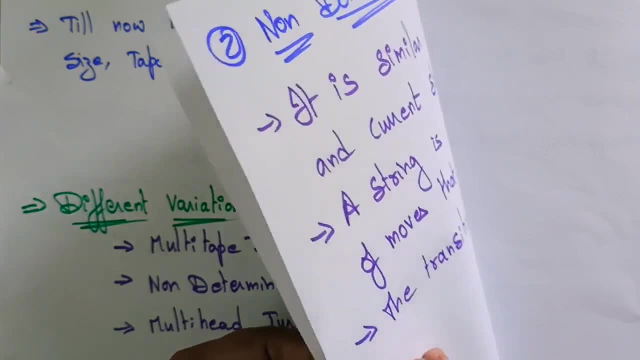 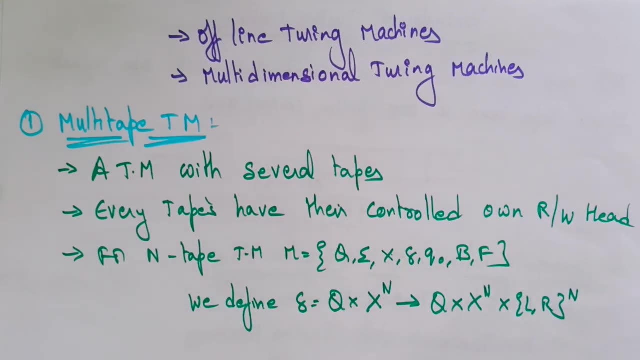 In the Turing machine and non-deterministic Turing machine. multi-head Turing machine means there are multiple heads that moves towards left and the right. multi-head Turing machine and offline Turing machine. and multi-dimensional Turing machine. So these are the different variants of the Turing. 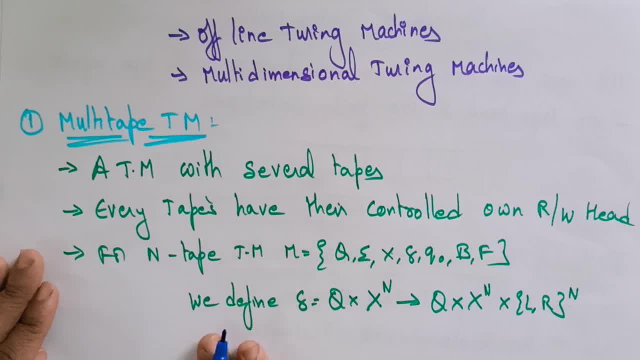 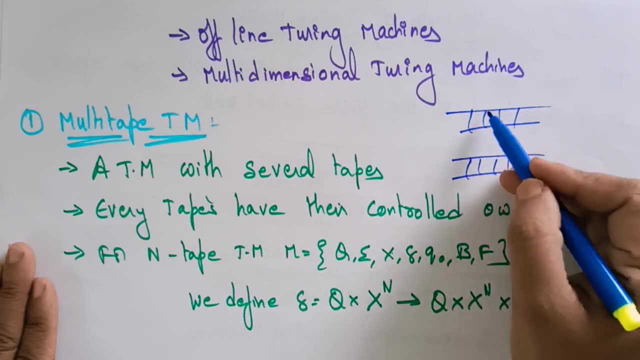 machine. Now let's discuss one by one. The first thing is a multi-tape Turing machine. Multi-tape means we are having the multiple tapes. This is one tape and this is another tape. Each tape is cells and there is a head pointing towards the tape that moves towards the left and moves towards 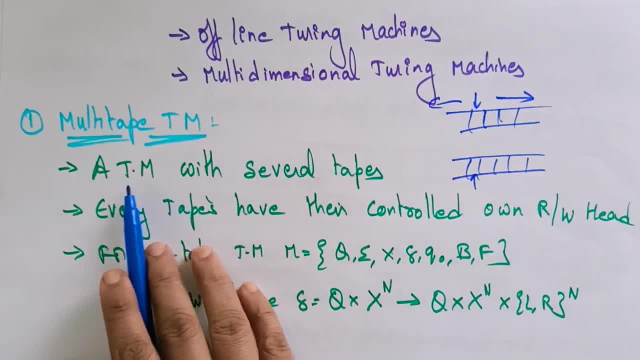 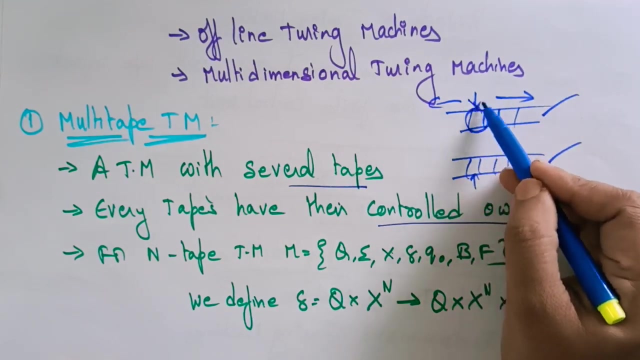 the right. that is a concept. okay. so a multi a turing machine with several tapes- you call it as a multi-tape turing machine- every tapes have their controlled own read or write head. so whatever the tape you are taken, so that tape is having their own controlled read or write head either. 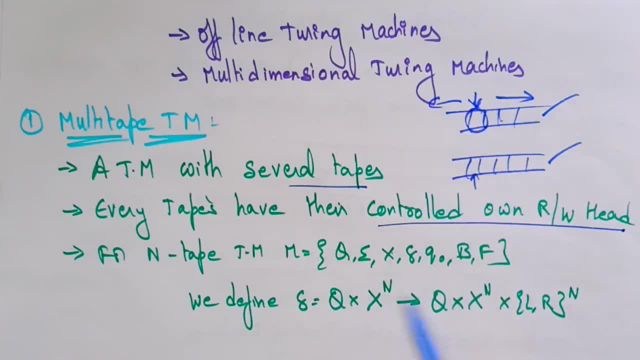 it can read or it can write head will be there. suppose for n tape of turing machine. let me take there are n number of tapes in one turing machine. so the equation, the formula, the definition for that is the turing machine m is equal to q, sigma x, delta, q, naught, b, f. so just like a turing machine. 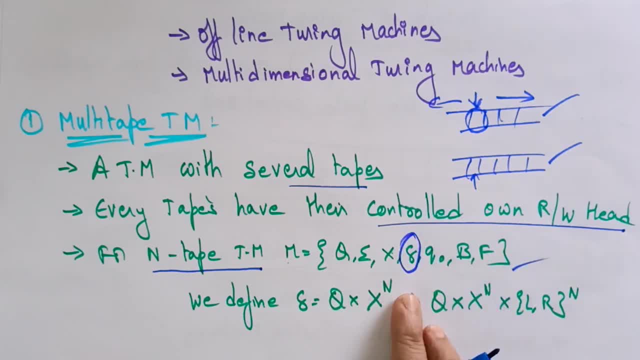 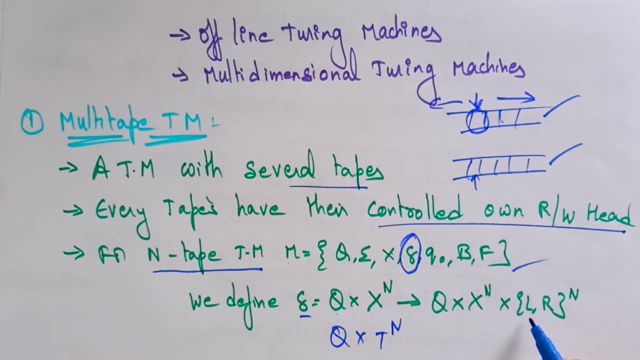 definition. but only thing is the transition function will be changed because here we are using the multiple tapes, so we define the transition function: is q into either. you can write q into t power n- okay. x power n. that implies q into x, power n into either. it moves to the left or right. how many times? n number of time power n: okay, because we are using 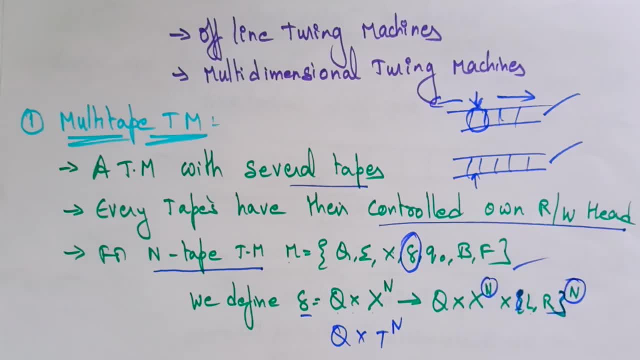 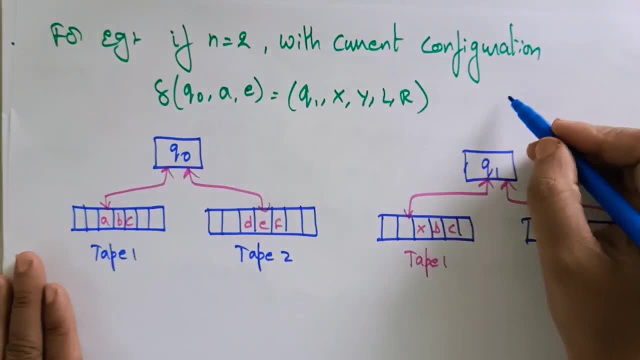 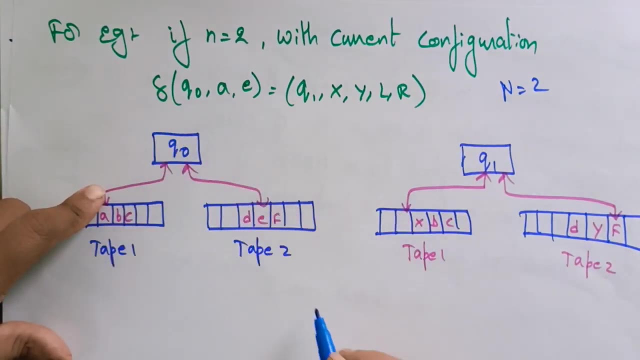 the n tape. so you just need to keep this power n if you are using the multiple tape. so see in this example: suppose if you are taking n is equal to 2. i have taken n is equal to 2 with the current configuration. then the transition function. so what is the transition function? i said q into uh, transition. 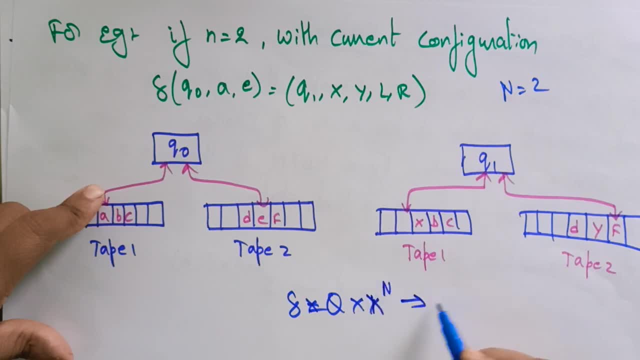 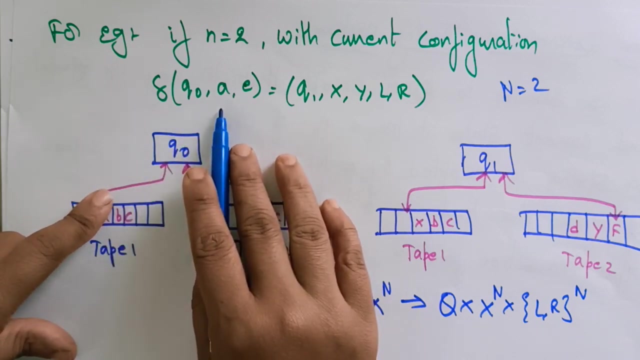 function is q into x. power n is implies q into x, power n into either. it can move to the left or right. power n: okay, so q is the state. what is the present state that we are using? okay, so the present state and the input alphabet: whatever we are taking, and e okay means i'm moving from uh. 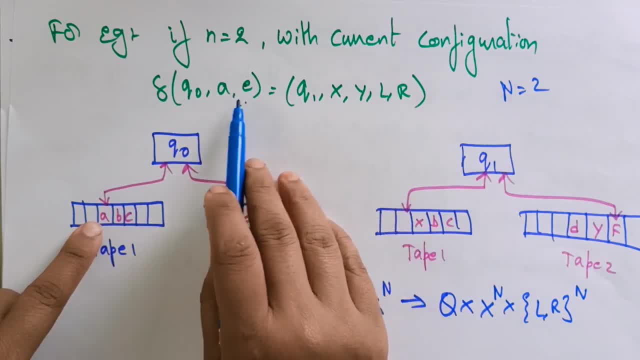 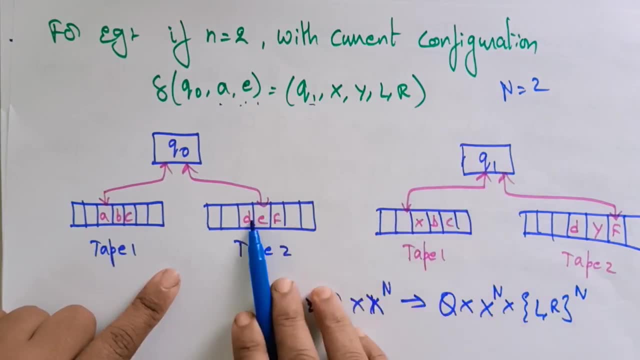 so the head is pointing towards uh, e. okay, a and e. so now here, q1 is the next state as the next state. okay, so this is one state. q naught with having the two tapes because n is equal to 2. i use in the two. 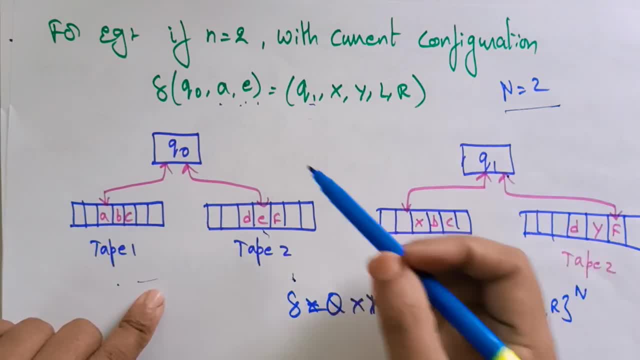 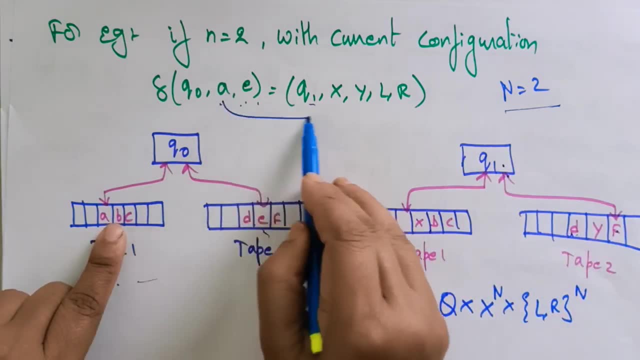 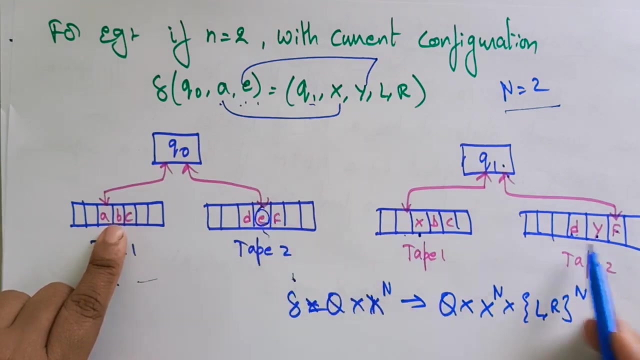 tapes, tape 1 and tape 2, and here the q1, which is the next state. in the next state, i am using the two tapes. okay, so there, a is replaced with a. is replaced with the x. okay, so this is the next state. and e is replaced with the y and the e. whatever the e is there, that is replaced with the y. 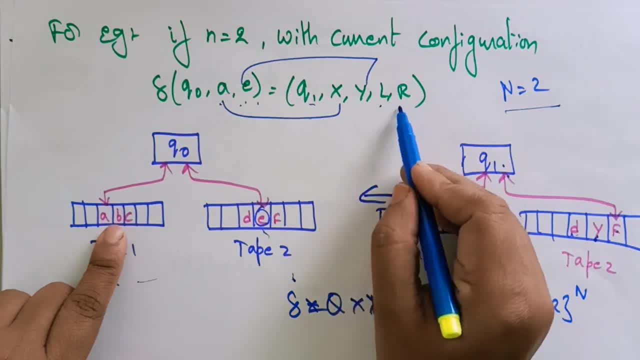 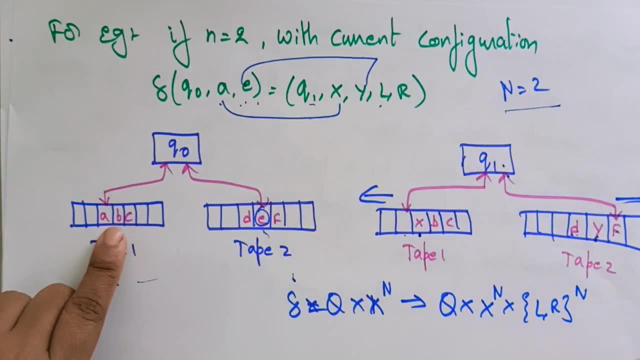 okay, and this is moves towards the left and here this point moves towards the right. that is the meaning of this equation, if you are using the multi-tape, means here this is the state, present state, okay, and a e or the pointing variables in the head. so what will be the next state? so a should. 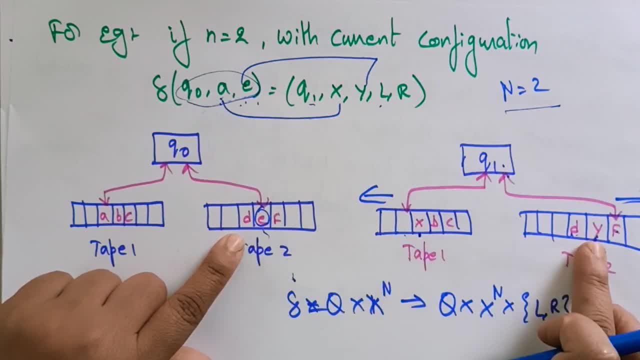 be replaced with the x, and e should be replaced with the y, and this tape moves towards left and this tape moves towards the right. this is the concept of the multi-taping or multi-tap turing machine. now coming to the next turing machine, the variance of